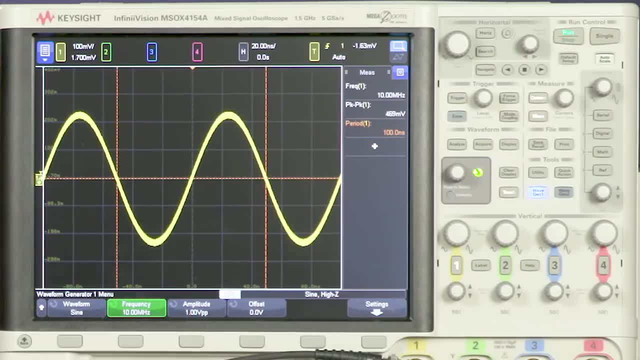 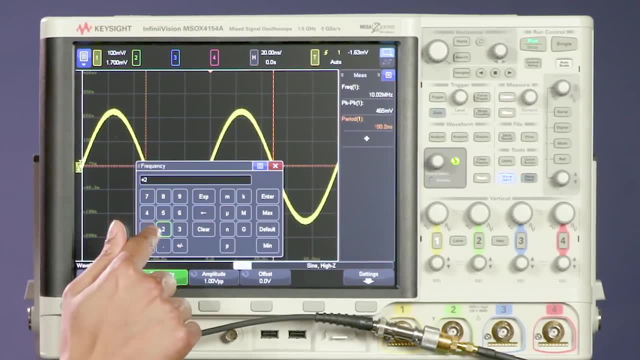 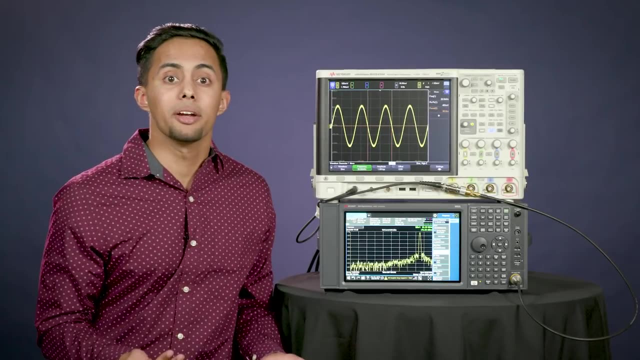 waveform with a period of about 100 nanoseconds. Now, if we were to adjust the output from the waveform generator to a 20 megahertz signal, then this is how it would look on the oscilloscope Once again as a sinusoidal waveform with a period of about 50 nanoseconds. Basically, the higher. 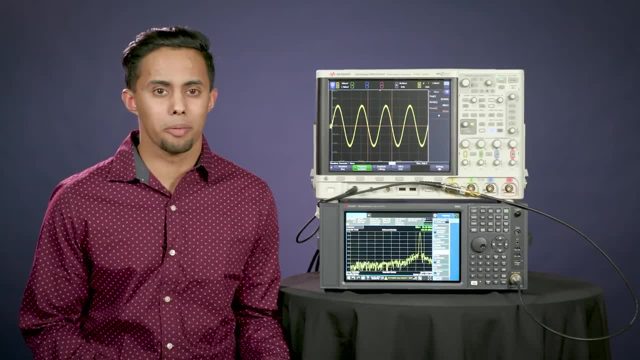 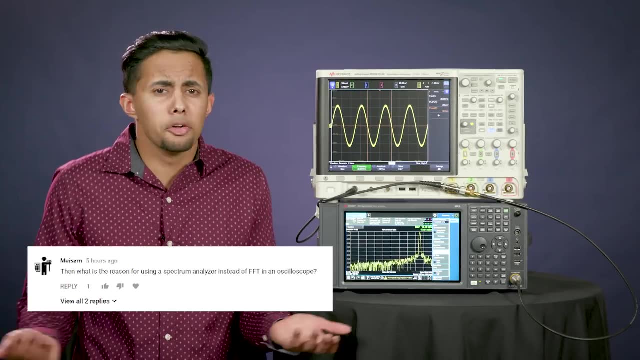 the frequency, the more waves we see in the same span on our oscilloscope. Now, in my last video I got a question from one of you asking what the advantage of a signal analyzer is if you already own an oscilloscope with built-in FFT. Well, I'm glad you asked. Signal analyzers have lower noise. 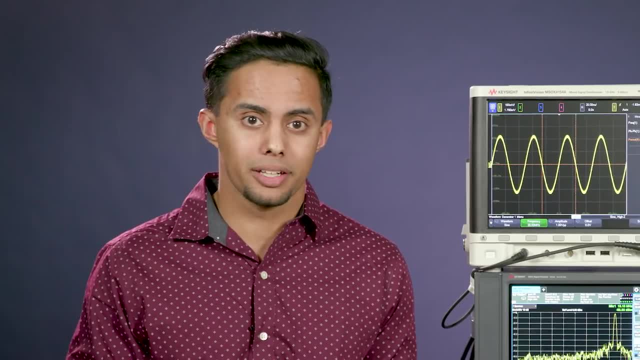 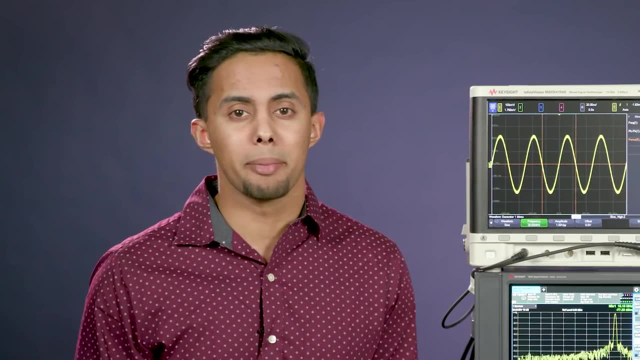 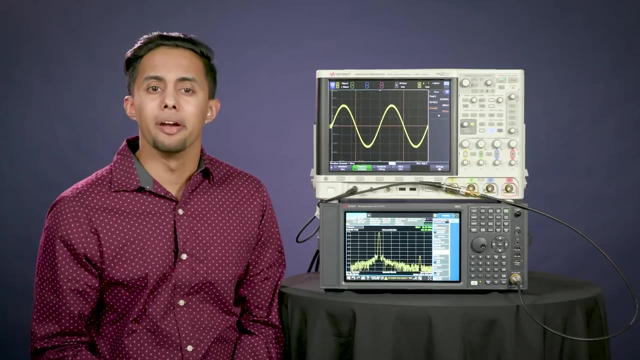 floors. this means they are much more sensitive to frequency components and are better at showing you low level signals. Signal analyzers also have better spurious free dynamic range, or SFDR, than oscilloscopes. All right, so now we have the signal analyzer and, as you may remember, signal analyzers. 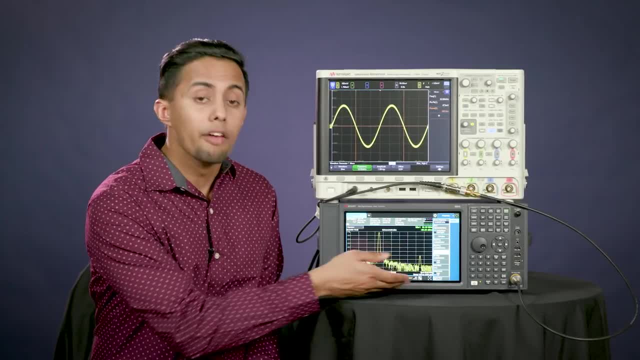 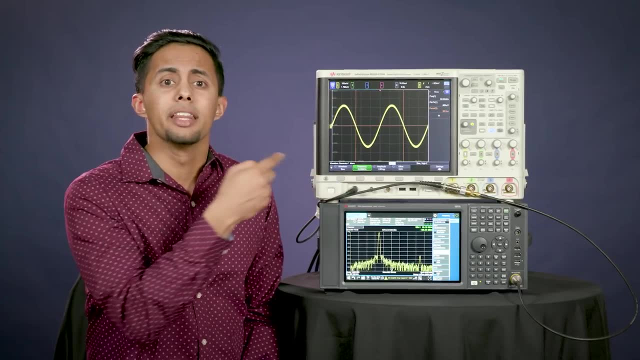 display signals with respect to frequency versus amplitude or the frequency domain. If we were to output the same 10 megahertz signal from the waveform generator that we had seen earlier on the oscilloscope to the analyzer, this is how it would appear visually: Just a single peak. 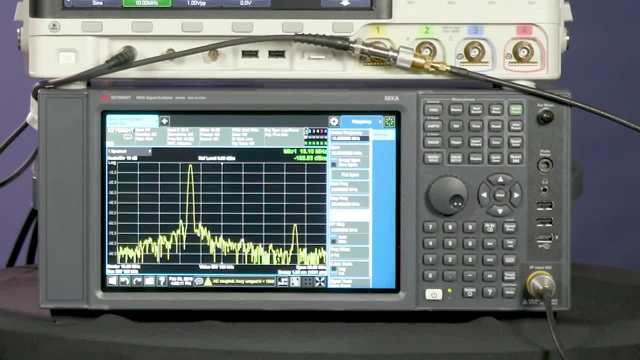 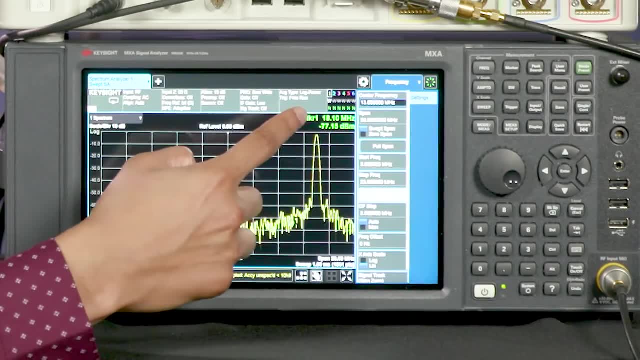 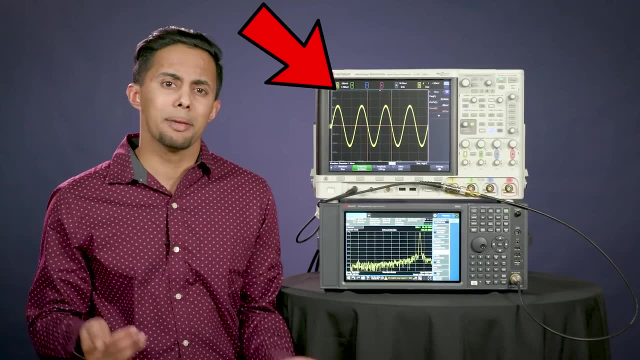 at 10 megahertz and if we were to just output the waveform generator to be a 20 megahertz signal, then it would be a peak that appears at 20 megahertz. So yeah, in the time domain signals appear as sinusoidal waves and in the frequency domain they appear as distinct impulses. 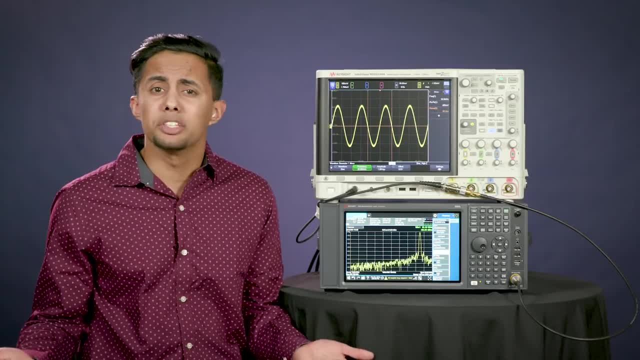 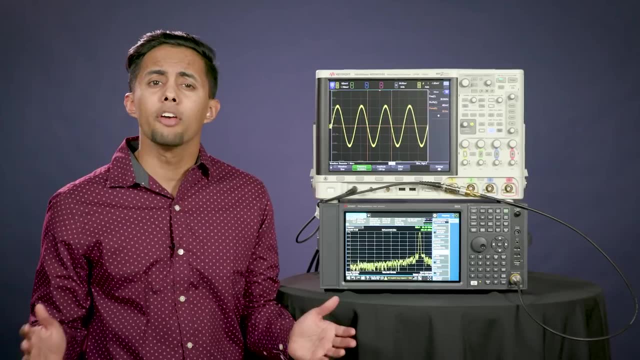 Okay. well, now this begs the question of why the heck do we care to use a signal analyzer? Is it just to show a wave as a line or something? Well, in a perfect world, we would see the sinusoidal waveform like the ones we saw on our oscilloscope at. 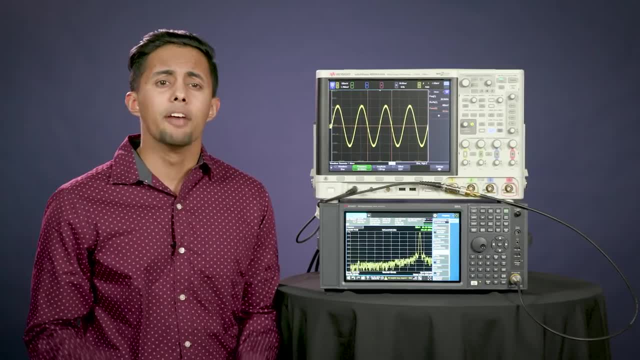 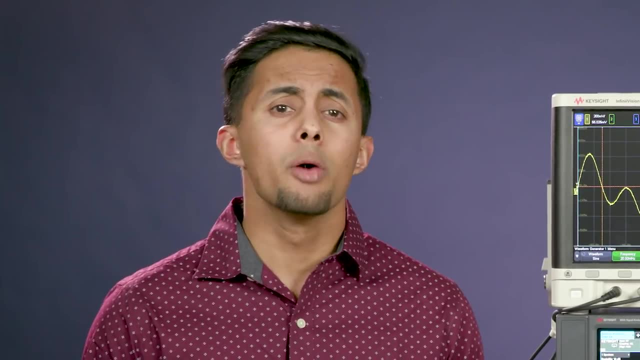 frequencies of 10 megahertz and 20 megahertz. Unfortunately, we don't live in a perfect world. When dealing with various devices, it's often you see a not so perfect sine wave with many ripples, like this one that I've now set up by feeding two sine waves from the waveform generator into 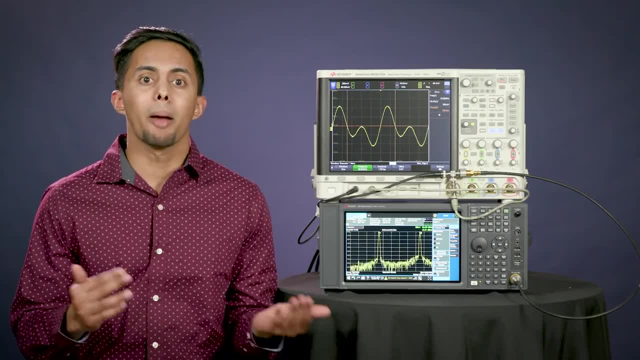 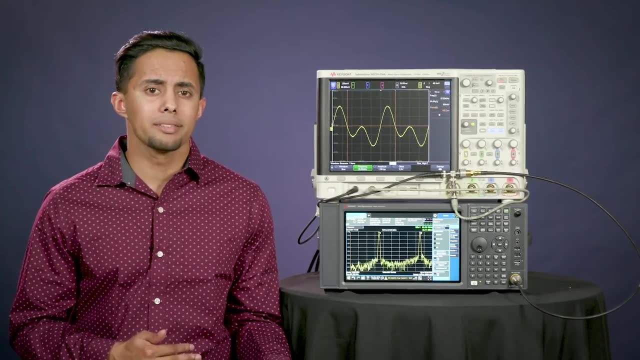 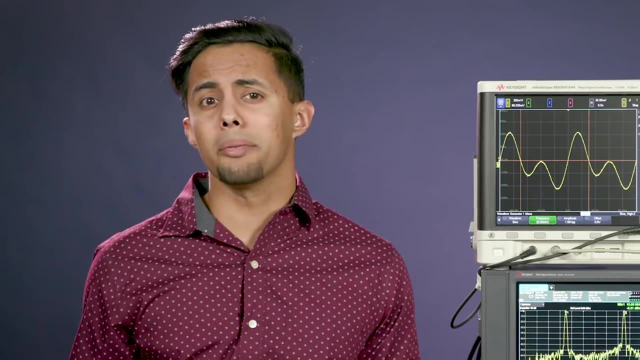 the oscilloscope, You could say that a real world signal can be represented as a sum of different sinusoidal signals, or rather different frequencies. Now let's say you're designing a product and your product can only operate in a specified bandwidth and it can't be emitting in other bandwidths. Then you must determine at what other frequencies 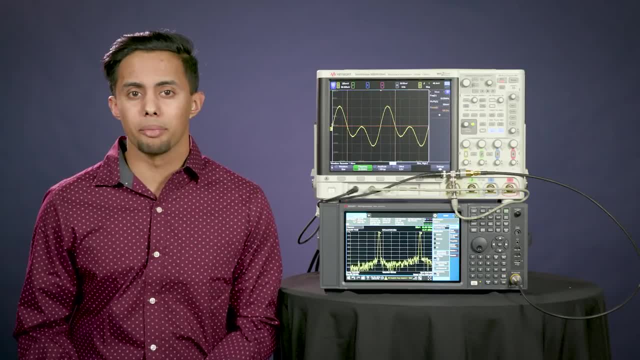 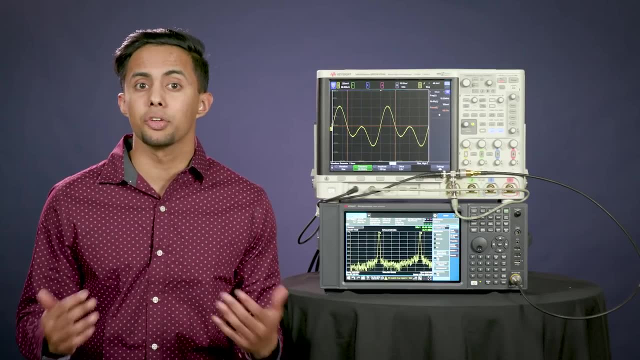 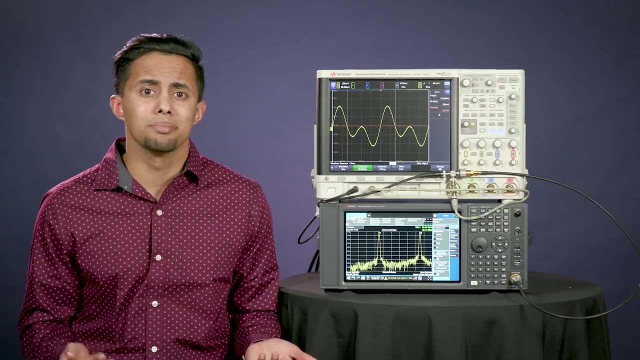 do the other signals exist that are corrupting the signal you want from your device, And that's where our signal analyzers come in. They help separate and display this combination of different sinusoidal signals into their distinct frequency components, So that if you were expecting your device to operate at, let's say, 10 megahertz, 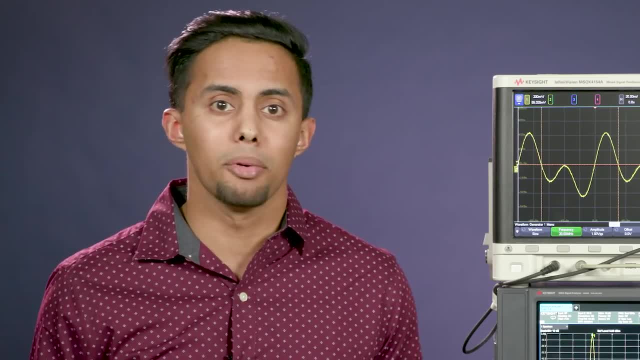 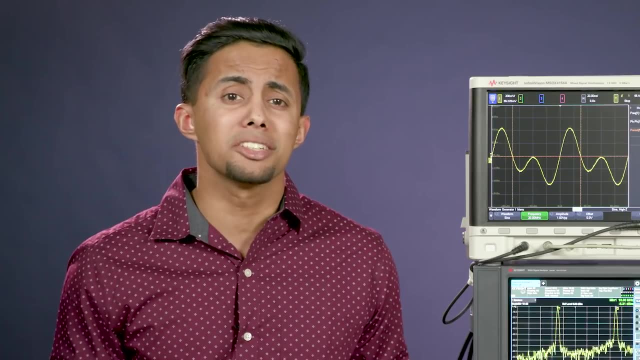 you can see all the other frequencies that are messing with your device, For example this 20 megahertz signal, And once that's figured out, you can use a bandpass filter to tune out those extra annoying signals you weren't expecting. All right, that's it for this episode. Thank you so much for watching. 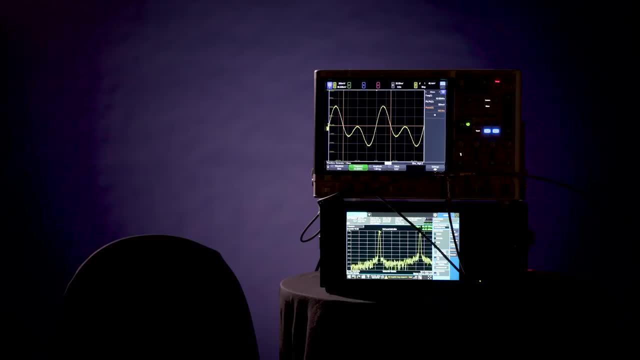 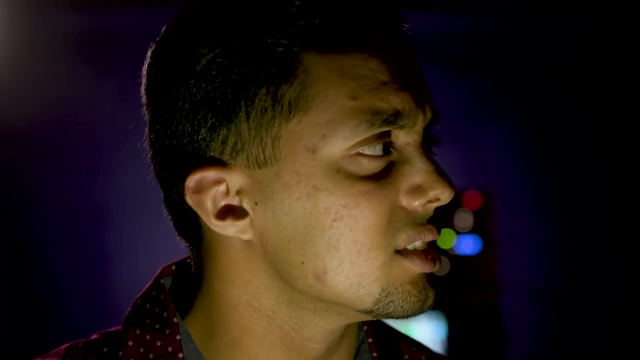